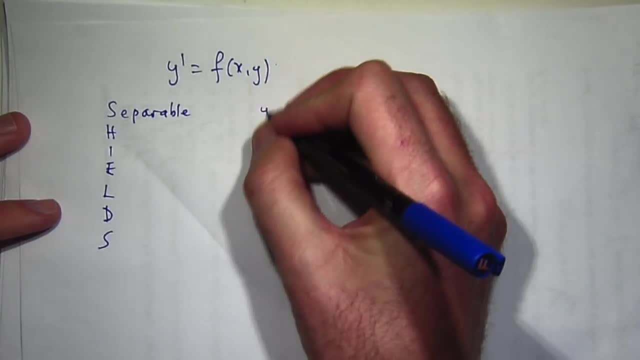 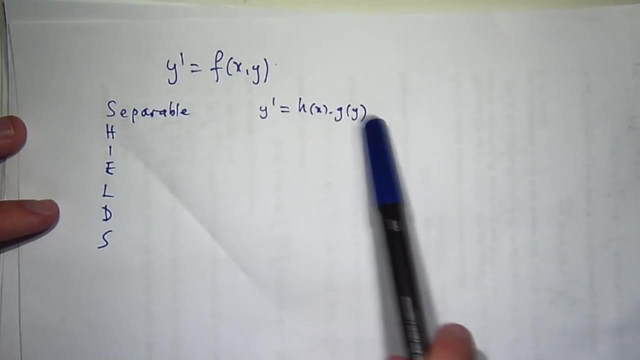 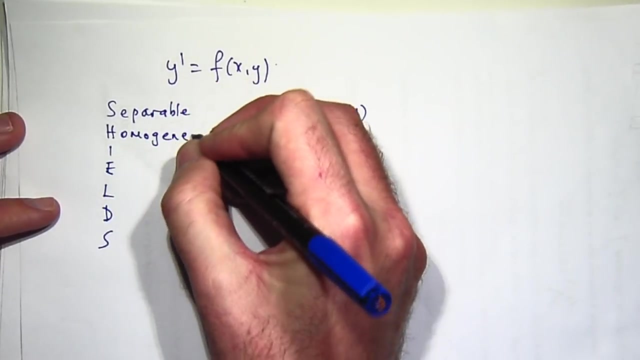 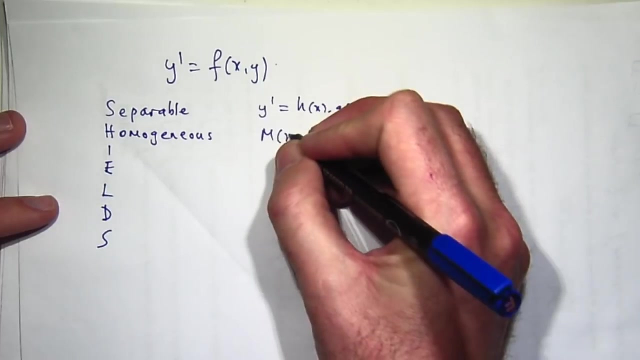 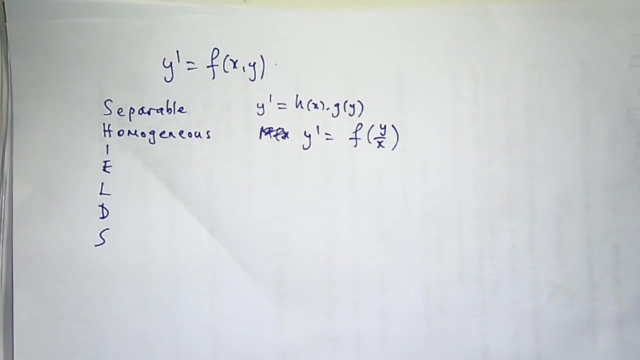 The differential equation might be separable. In other words, it's something like this: Okay, You separate the variables and you integrate. Okay, So you have a special structure. Okay, In here you make the substitution: u equals y over x. 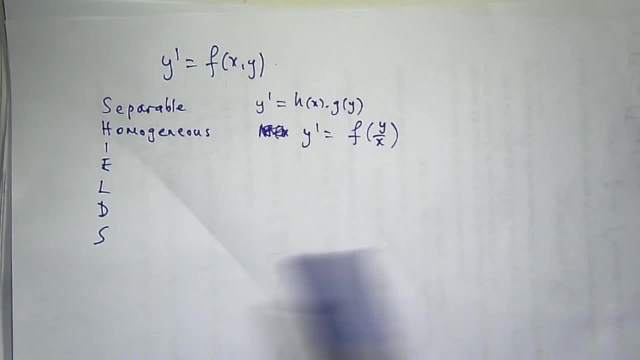 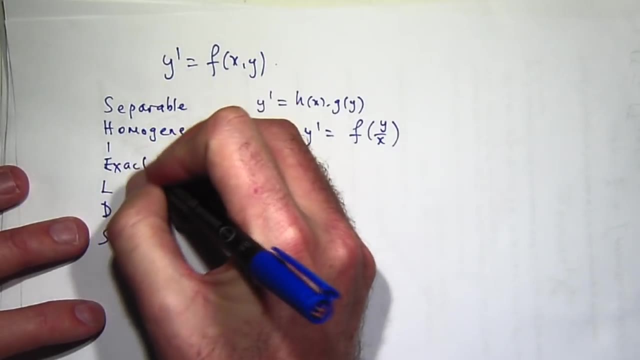 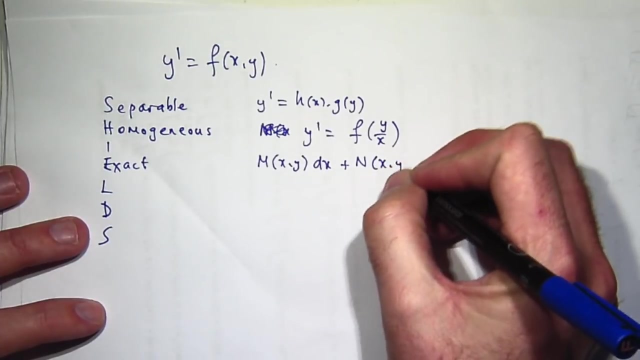 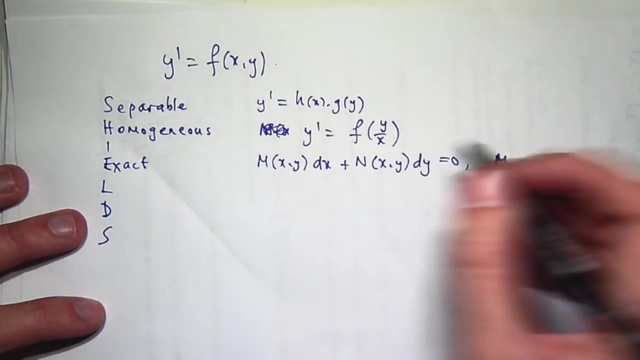 And then you form a separable differential equation. Now I'll leave the i for a minute. What do you think the e stands for? Exact Right. So that's of the form, Usually, where the differentials are separated and you have the partial derivatives of these m and m, satisfying some sort of relationship here. 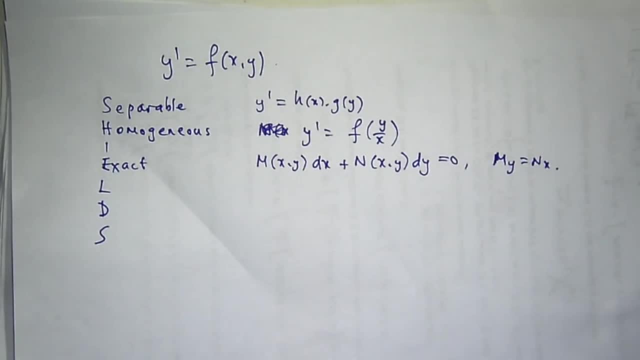 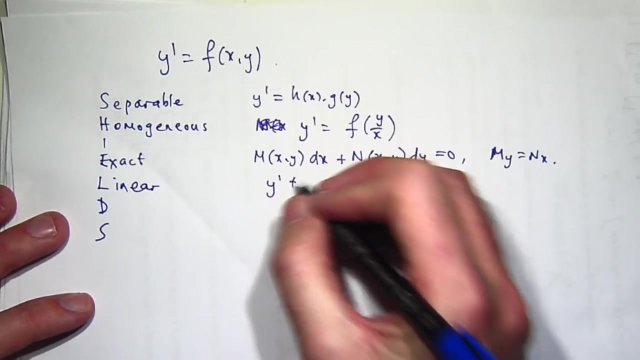 By the subscripts I mean partial derivatives. So m sub y is dm dy with curly d. m sub x is dn dx with curly d. What do you think the l stands for? Linear, Linear Right. Okay, So that's when the equation is of the following form: 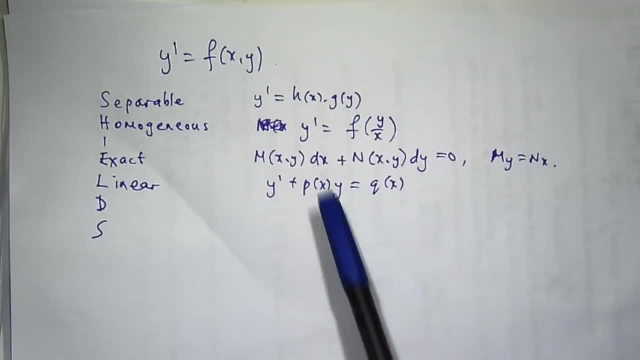 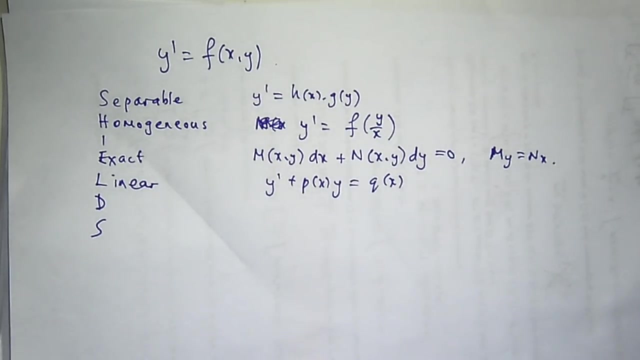 Okay, So to solve a linear equation, what you do is you look at this coefficient function of y And you form an integrating factor e to the integral of p of x, And you multiply through both sides, And then you use the product rule to reduce the left-hand side to the derivative of the product. 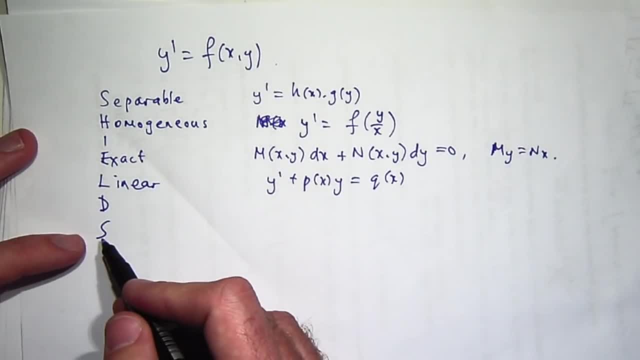 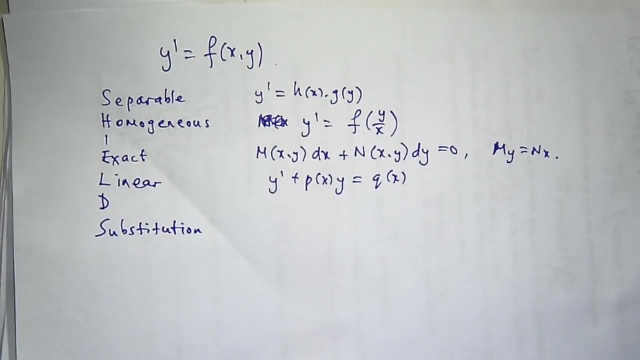 Okay, I'll leave d for a minute. What do you think s stands for? We've already used separable. What's another way to solve a d? Well, via substitution sometimes. Okay, So you can take a very complicated differential equation, possibly a non-linear form. 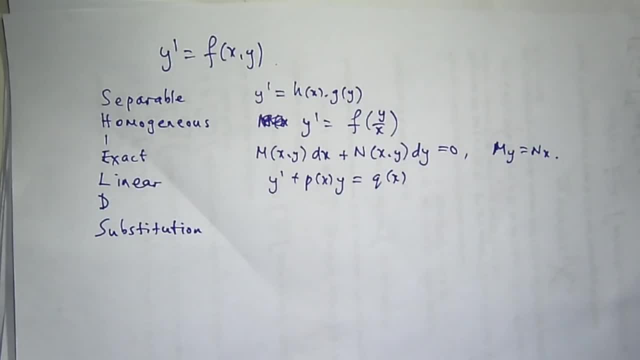 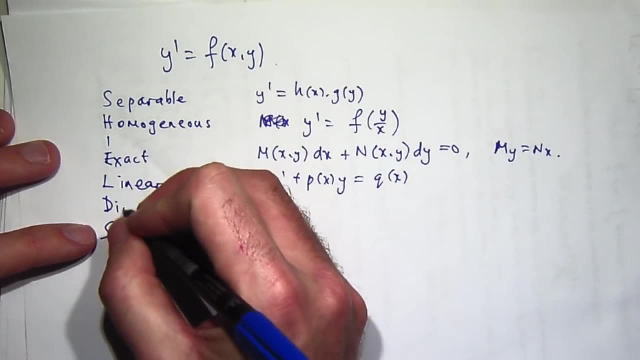 And, for example, Use a certain substitution to reduce it to a linear form. Okay, Sometimes There are lots of other substitutions. Now, by the d here I mean you can solve the differential equation directly, In other words, just by direct integration.